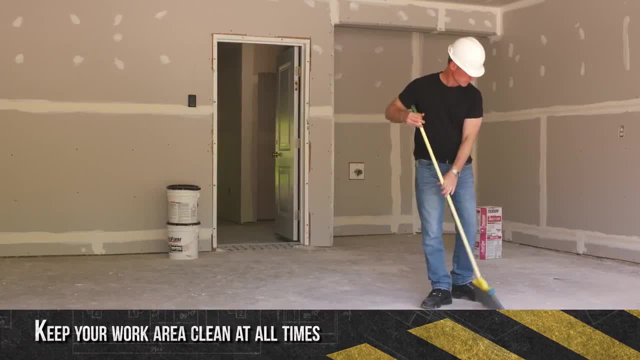 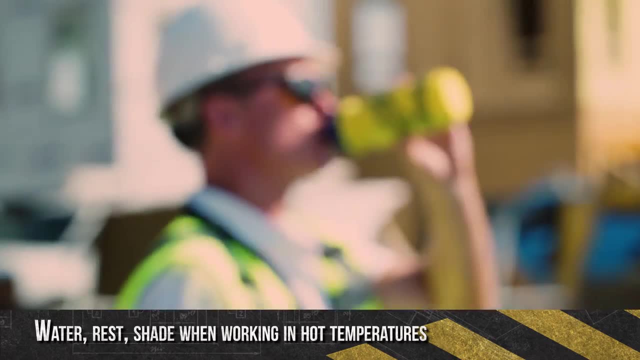 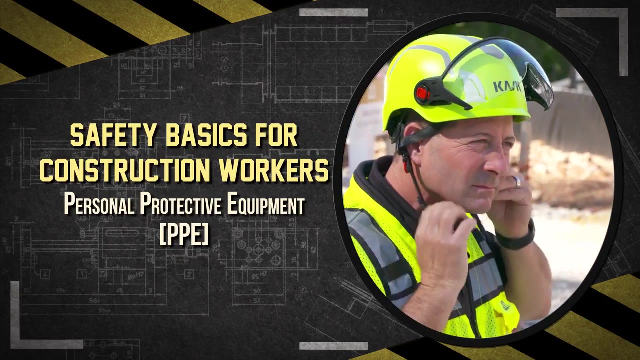 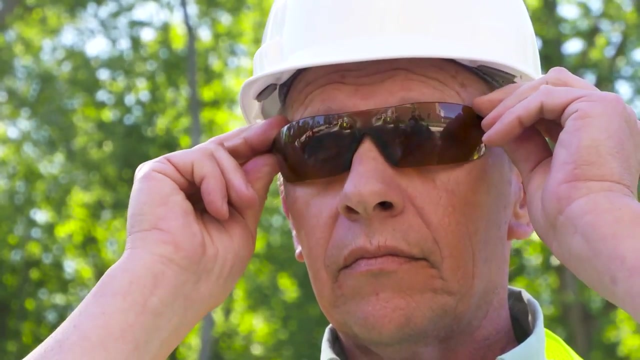 walkways and stairs clean and free of trash. They must use the appropriate tools and materials to prevent tripping and take adequate precautions when working in very hot temperatures, including frequently drinking cool water and taking breaks in the shade. Personal Protective Equipment, or PPE, is designed to protect workers from serious workplace. 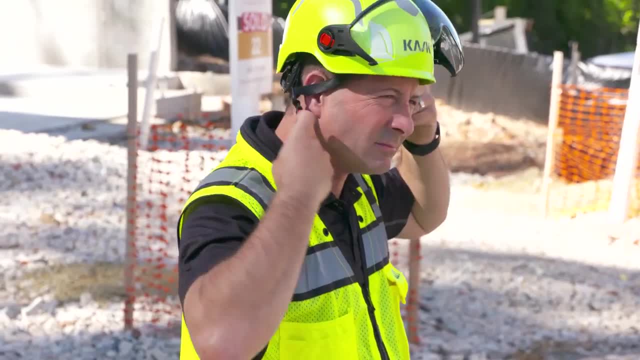 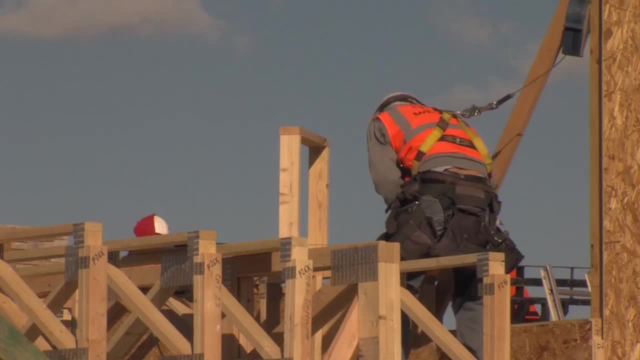 injuries and using PPE is essential. Always use the appropriate equipment. Make sure you have the appropriate PPE, such as wearing a hard hat, safety glasses, safety boots and gloves, as well as high visibility clothing and hearing protection, and even. 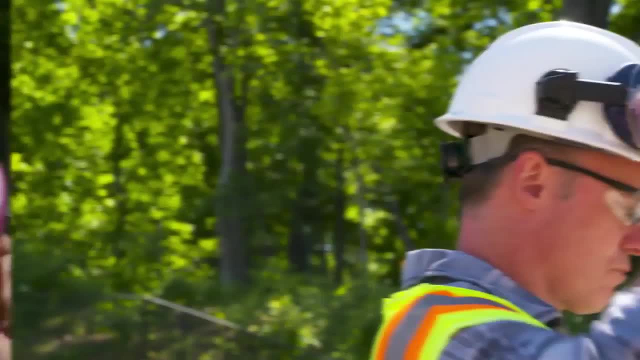 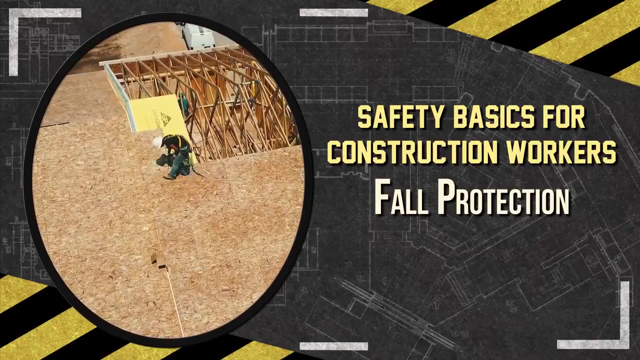 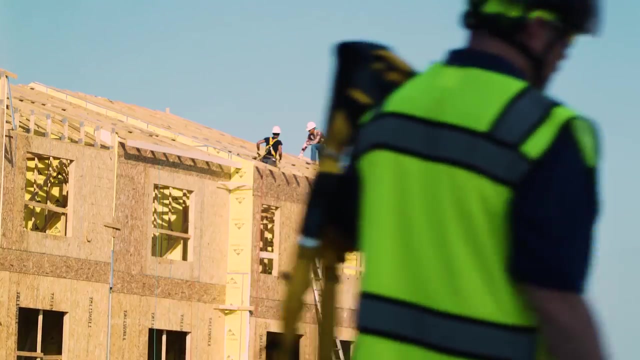 respirators when required, in the manner that they were designed, Ensure the PPE is maintained in good condition and replaced when damaged or lost. Falling is the number one cause of serious work-related injury and death in construction. The best way to prevent a fall is to inspect the work area and ensure all fall exposures. 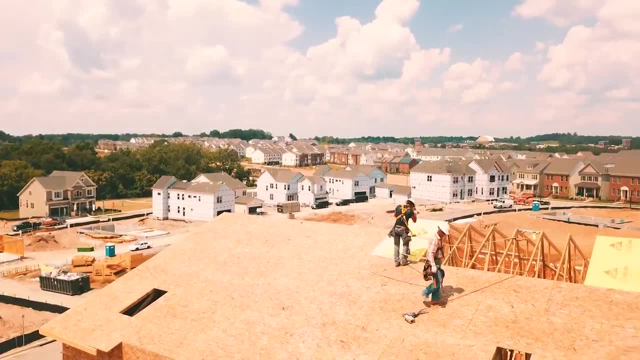 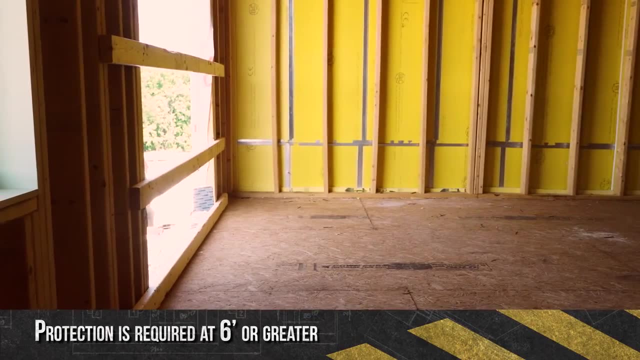 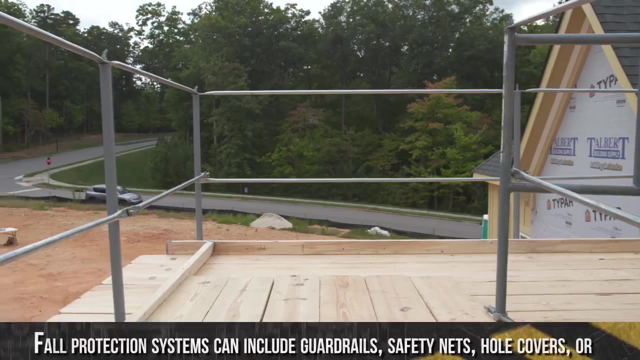 are adequately protected. Workers exposed to fall hazards six feet or more above a lower level, such as a leading edge, floor holes or wall openings and roofs, must be protected by a fall protection system. Fall protection systems can be temporary or permanent. guardrails, safety nets, hole covers. 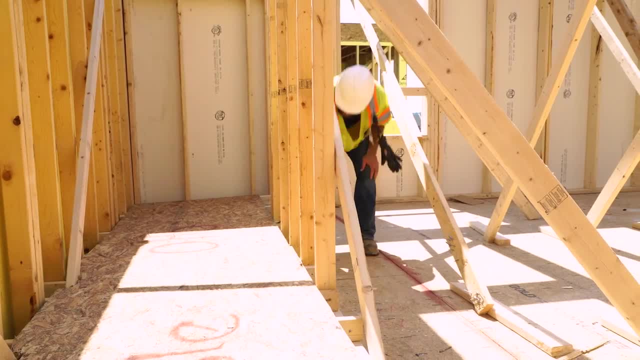 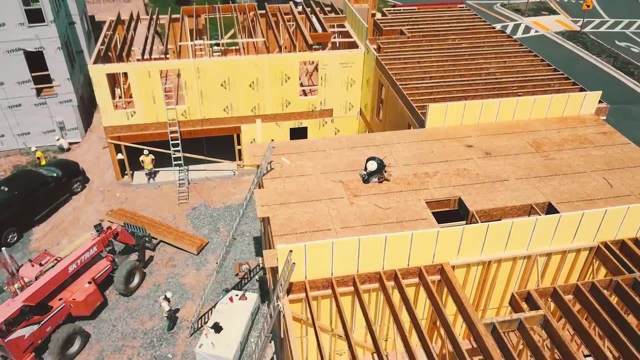 or personal fall arrest systems. A competent or qualified person must oversee the installation of the fall protection systems. For more information, visit wwwFallProtectionSystemsca. Don't work around unprotected floor and wall openings or skylights, and never walk the. 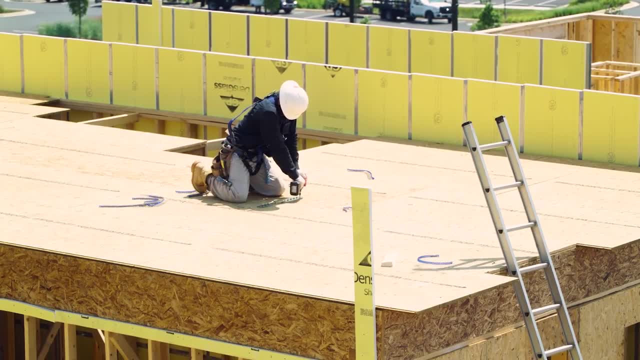 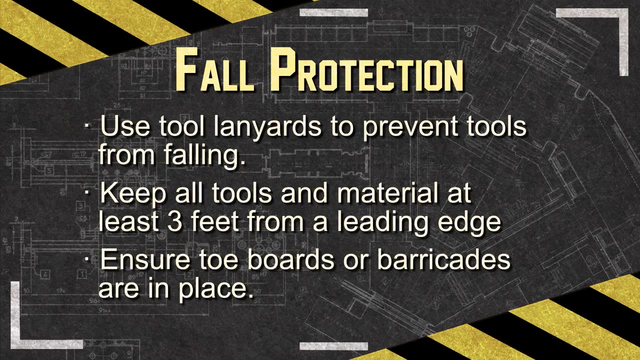 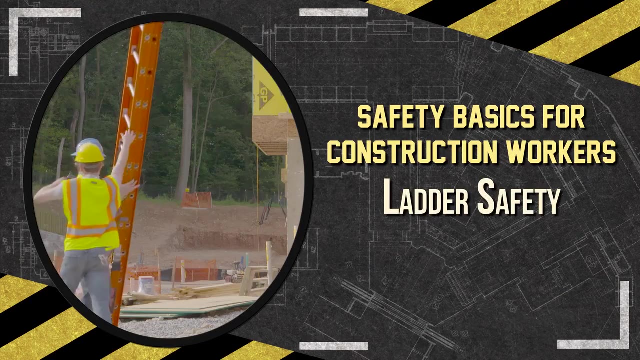 top plate of a wall unless using the right fall protection equipment. Protect workers from falling objects by securing all tools, equipment and materials when working on an elevated surface or restricted access to areas where a fall or drop hazard exists. While it appears non-threatening, a ladder can be a major hazard. Ladder safety starts. 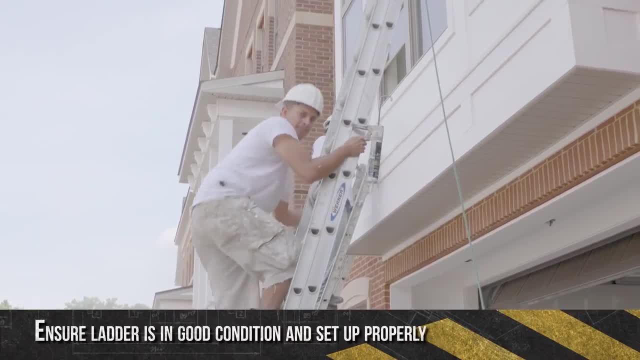 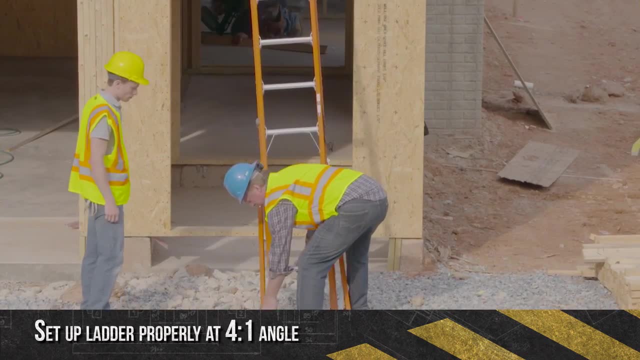 with choosing the right ladder for the job, Ensuring it is in good condition and in a proper position For extension ladders. set it on a stable, level surface at the proper angle. Extend it three feet above the landing surface to provide a handhold and secure it at the top. 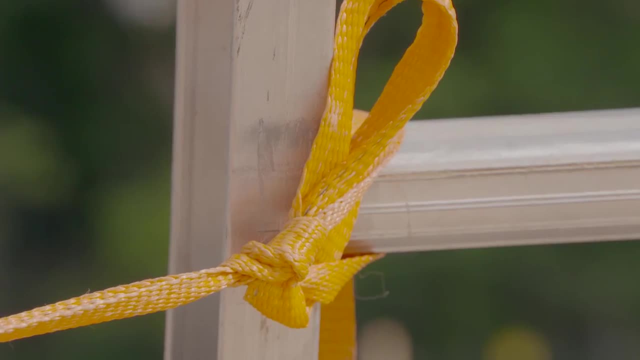 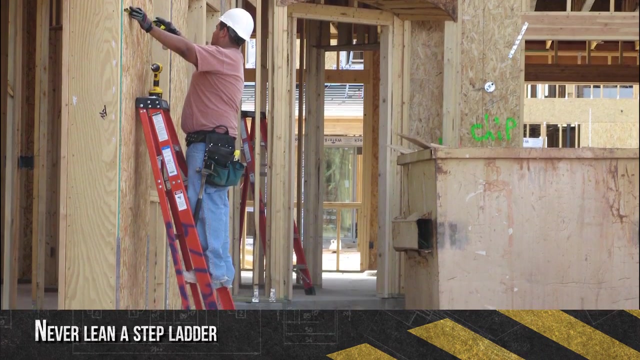 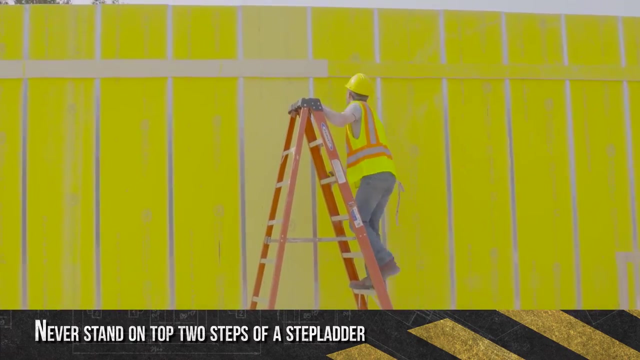 or bottom to prevent movement. When using step ladders, always set it up per manufacturer's instruction. Never lean a step ladder unless the manufacturer has designed it for that purpose and never stand on the top two steps of a step ladder. When climbing, face the ladder and maintain three points of contact. 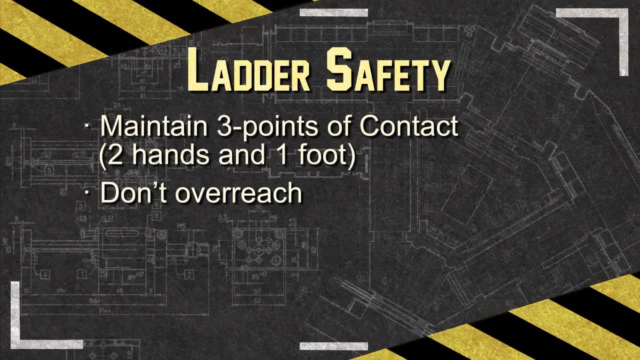 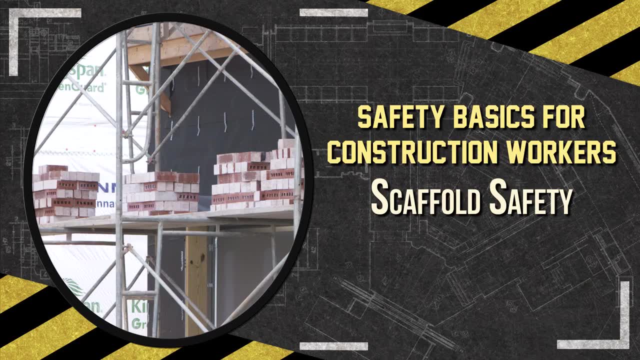 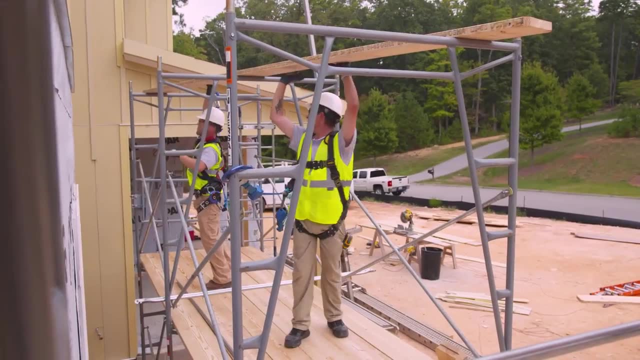 And remember, when working on ladders, don't overreach. Some workers will need to work on scaffolds, so you must be trained and understand the hazards before setting up, using or dismantling scaffolding. Don't work from anything not designed for that purpose, such as standing on a five-gallon. 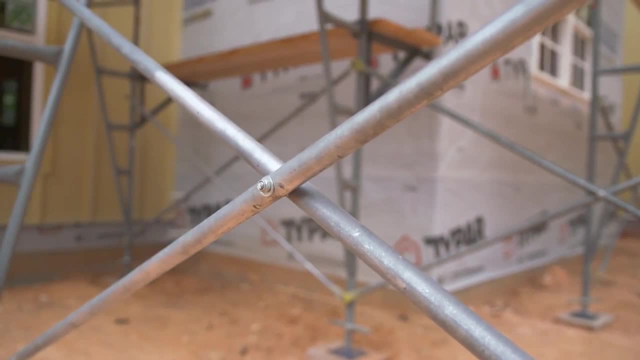 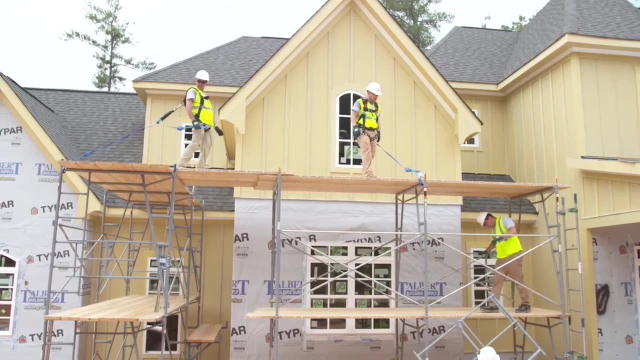 bucket, Because makeshift scaffolds are never acceptable. Scaffolds must be erected, dismantled and inspected before use under the supervision of a competent person, And for scaffolds ten feet and higher you must add guard rails or wear a personal fall. 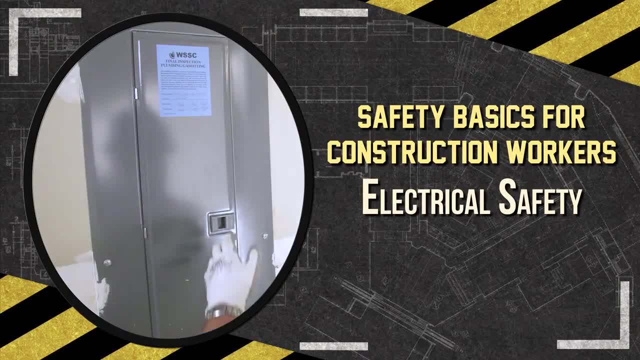 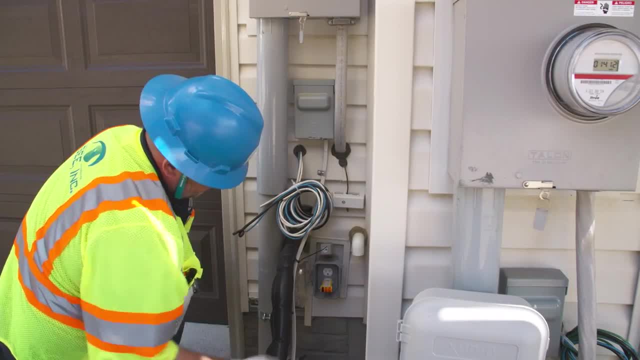 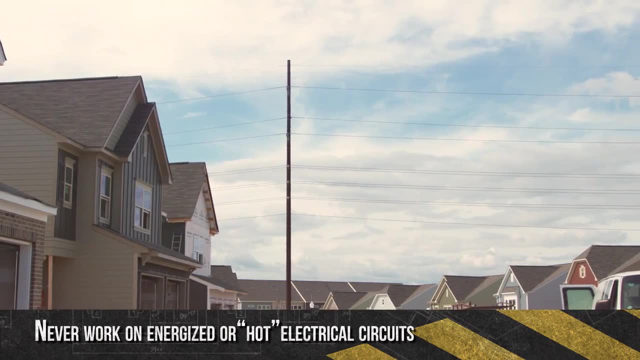 arrest system. Electricity can be extremely dangerous and can cause burns, shocks and death from electrocution. Anyone working with electricity must follow basic safety rules: Never work on energized or hot electrical circuits until all the power has been shut off and locked and tagged out, and remember to stay at least ten feet from overhead power. 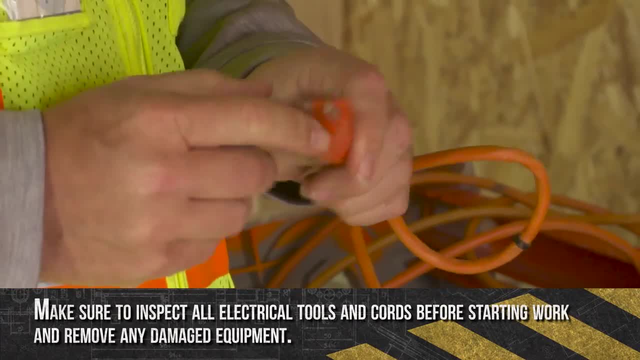 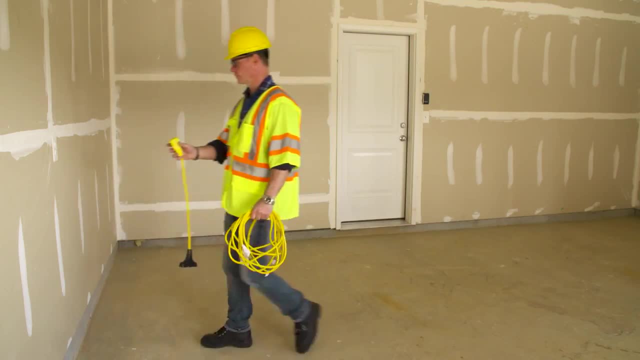 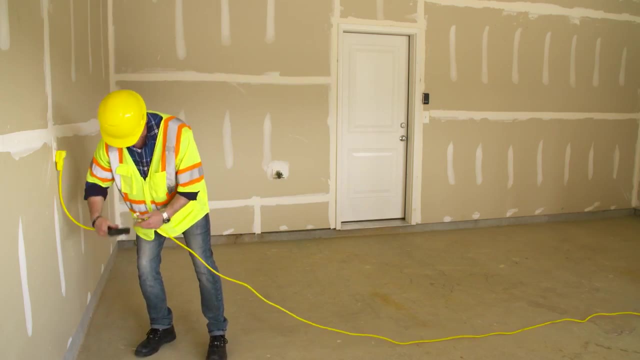 lines. Make sure to inspect all electrical tools and cords before starting work and remove any damaged equipment. Protect temporary power, including all extension cords and generators, with approved ground fault circuit interrupters or GFCIs, to protect against shock. And always use caution when working near electricity. 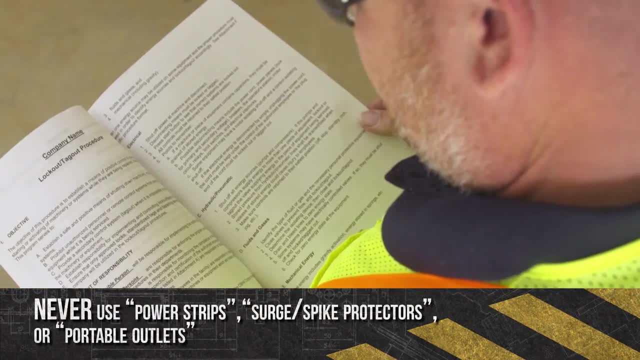 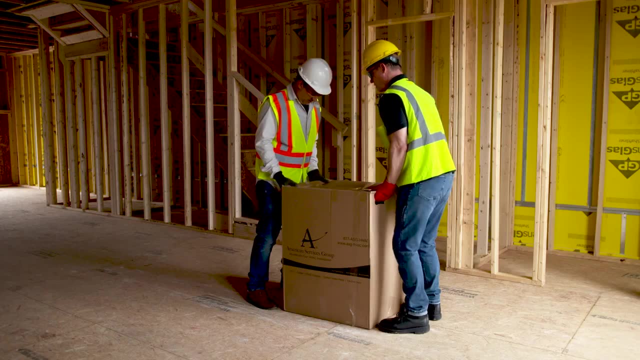 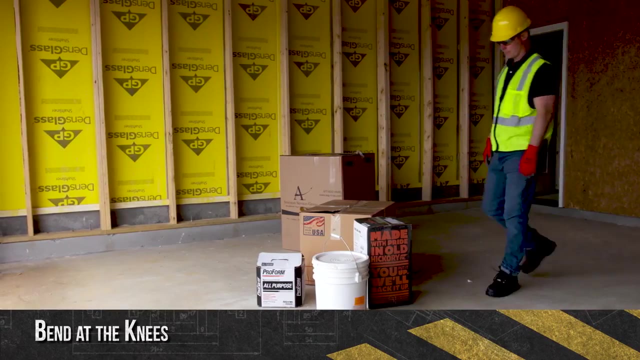 And never work on electrical circuits. Never use power strings on the job site. Using proper lifting techniques when handling heavy materials, tools and equipment can prevent back injuries. First, do not lift anything over 50 pounds without assistance. Next, bend at the knees as you lift the load, keeping it close to your body. 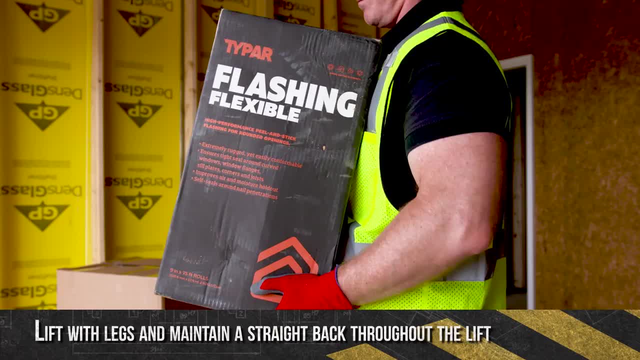 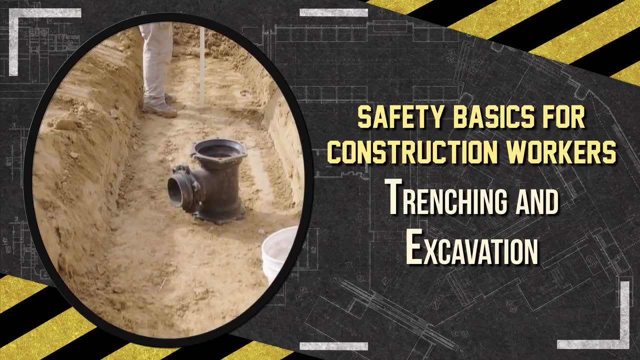 Lift with your legs, not your back. Finally, be careful not to twist your body during the lift. Cavens pose a great risk to your health. If you have an accident, you may need to check your health. If you do not have a life-saving device, you may be at risk.